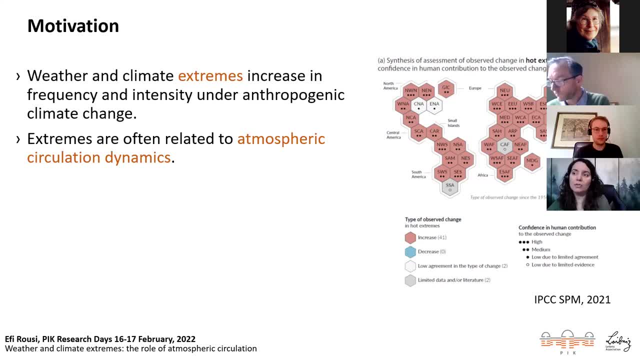 how and in how much are those extremes related to atmospheric circulation dynamics? On one hand, there are. there are the thermodynamics, which are simpler to understand and to model, but the atmospheric circulation dynamics are more complex And, according to the same report of IPCC, there is low confidence in how dynamic changes have affected and will affect the location and 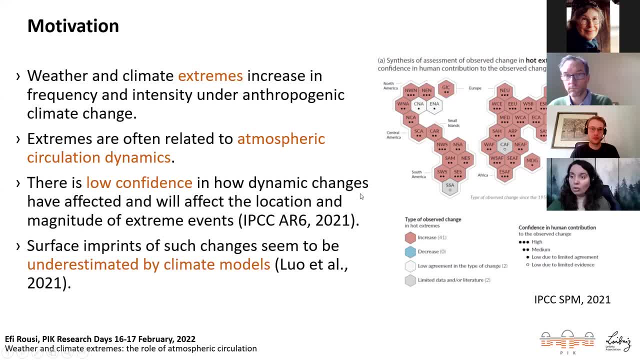 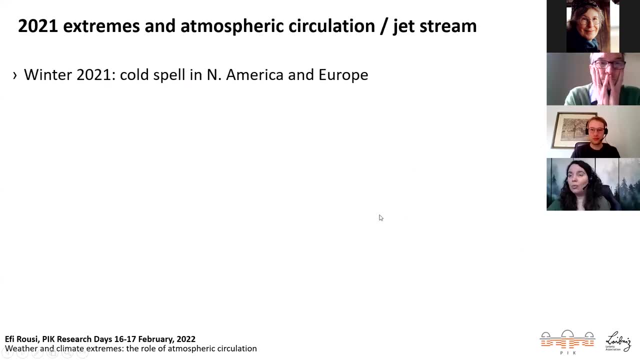 magnitude of extreme events, And we also know from recent research that the surface imprints of such changes are underestimated by climate models. This actually links very well also to the talk given earlier by Peter Hoffman, So I would like to show you a few things about some of the extremes that 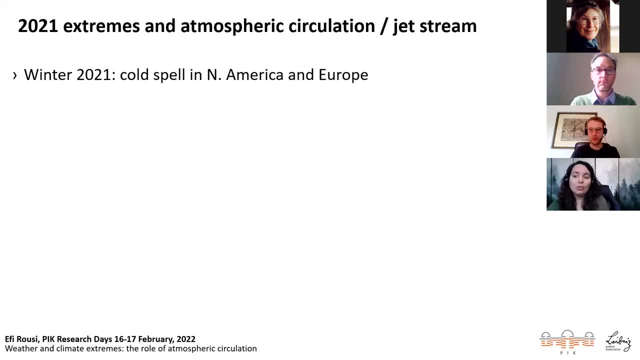 we saw last year, in 2021, that have to do in some way with atmospheric circulation and jet stream configurations. For example, starting with the winter 2021, we had this particularly cold spell in North America and Europe, which was linked to a disruption of the stratospheric polar vortex. 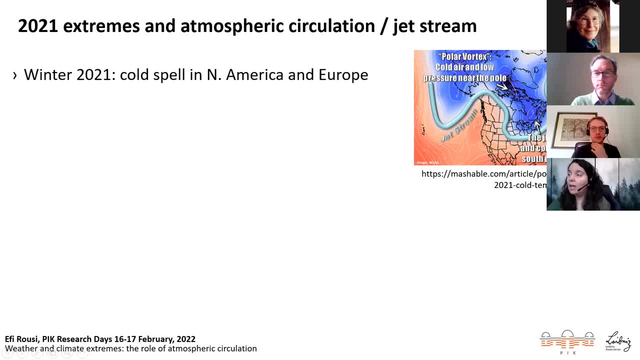 This in turn influenced the jet stream in the troposphere that was particularly wavy- or meandering, let's say- And this allowed for cold, cold polar air to go to high, to lower latitudes and central US and southern US states, causing many disruptions. And we saw this cold wave also in Europe. Later in summer, in June 2021, we had an extreme heat wave. 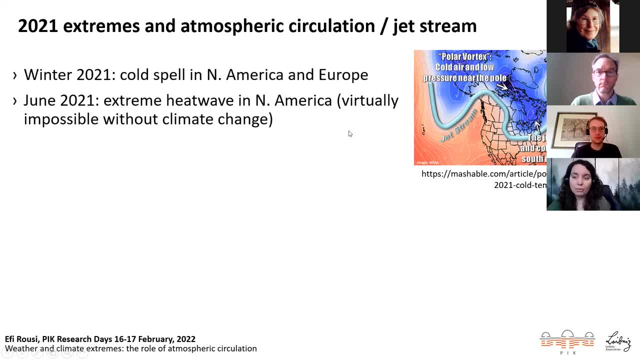 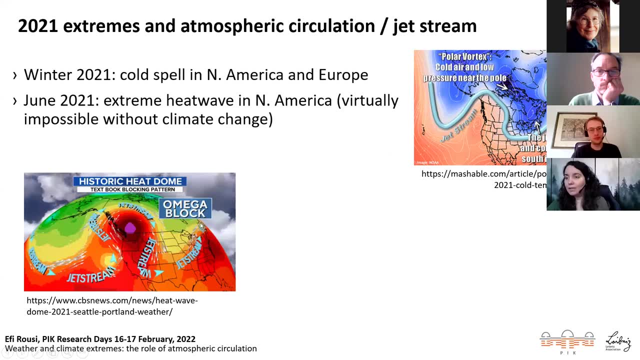 in Northwest America which, according to an attribution study that was done afterwards, was virtually impossible without climate change And this is a very important point- Anthropogenic climate change, and this is a characteristic figure from CBS News. They called this a historic heat dome. Heat dome is another way to refer to a blocking high. 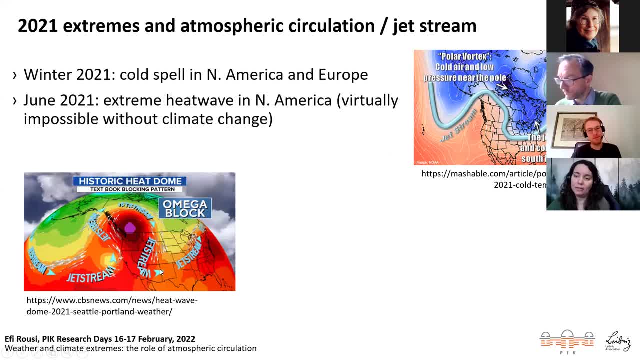 pressure system. practically, This is again an omega block, similar to what we also saw earlier from PETA, And this blocking high system stayed in place for a long time, causing extreme heat and drought in the region and coming closer to us spatially. we, of course, had the 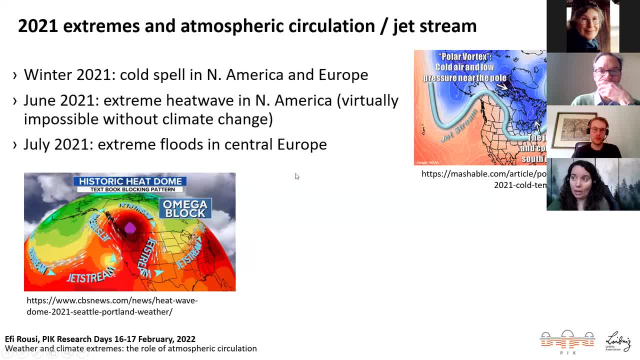 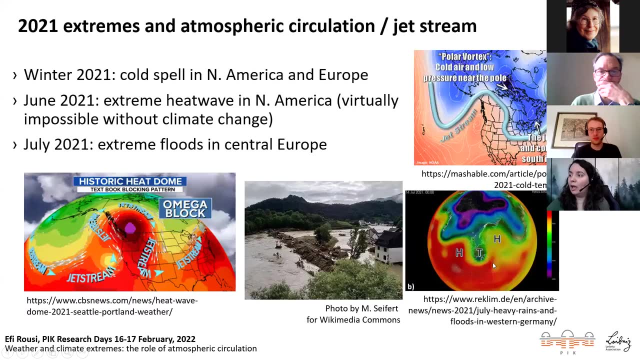 extreme precipitation and catastrophic floods in July 2021 in Central Europe, Western Germany and the surrounding regions. And of course, this is also related to atmospheric circulation patterns and to the jet stream And, for example, this was characterized by a cut-off. low, sorry, so a low. 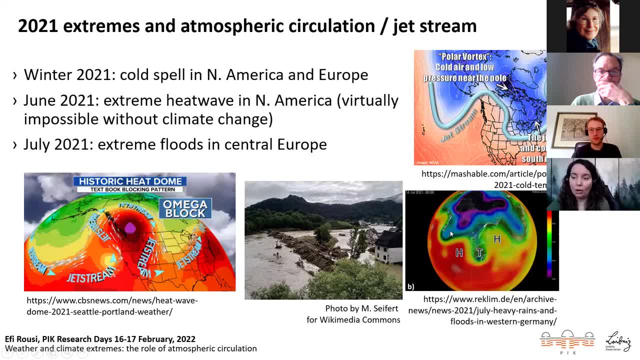 pressure system that was not embedded in the normal, let's say, flow of the jet stream, which was positioned in a northern position compared to climatology this summer. I will now show you some of the results of my current work, which are currently in revision in Nature Communications. 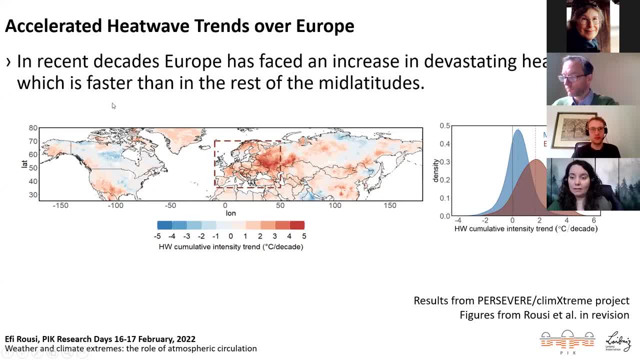 And these have to do with heat extremes and jet stream configurations for Europe. So we know that in recent decades Europe has faced an increase in devastating heat waves And in this work we tried to quantify this increase and compare it to other regions, And we found that the increase in 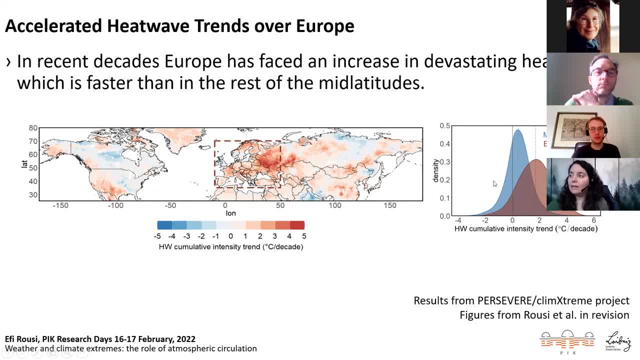 Europe is faster than in the rest of the mid-latitudes. We can see that in those two figures. On the first one on the left-hand side, we see for each grid point of the mid-latitudes the trend of heat wave cumulative intensity in degrees Celsius per decade. And indeed we can see that many regions of Europe 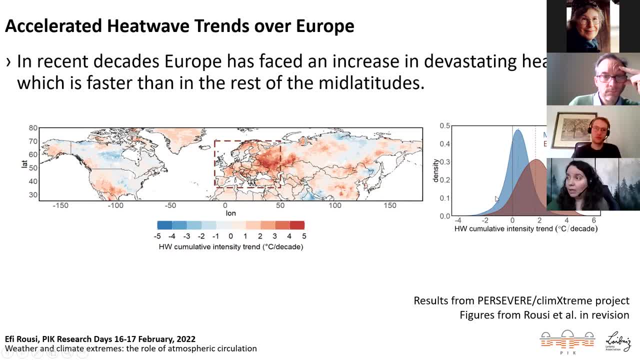 present hotspots And on the right-hand side we have plotted the distributions, the PDFs of those trends for all grid points of the mid-latitudes and all grid except excluding Europe with blue color And the grid points over Europe, as seen in this extended European domain, as seen in this box. 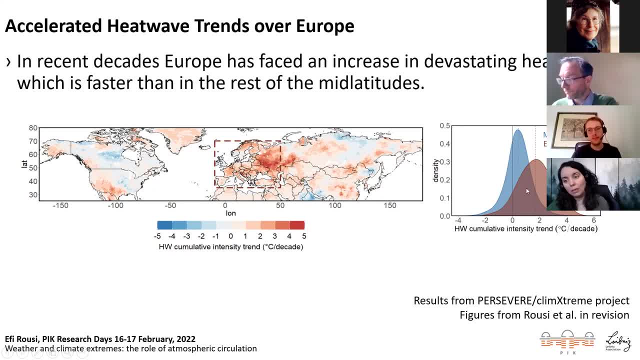 in brown And we see how the distribution for Europe is shifted to much larger values. And if we look at the mean which is plotted with these numbers here, the mean over Europe is almost four times the mean of the mid-latitudes. But the question is why is this happening And whether there are some links. 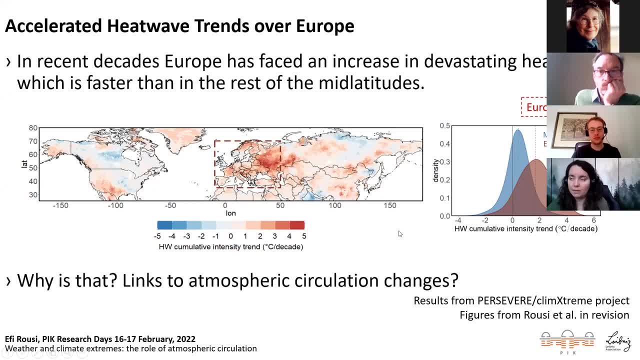 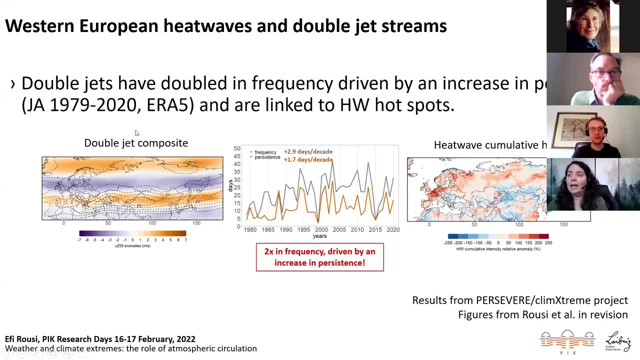 to atmospheric circulation changes that can explain this difference. So, in order to answer this question, we looked at jet stream states and we found that a composite, a cluster of double jets that look like this first figure. So here we see, the anomalies of the zonal wind at the 250. 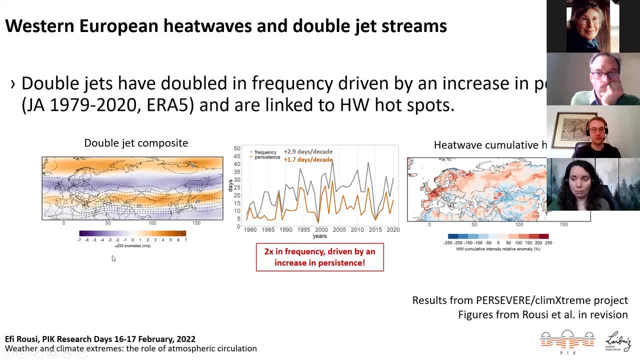 hectopascal level, which is near the tropopause where the jet stream blow, And we see that there are two zones of positive anomalies. so increased winds in the northern and southern location and in between, over northern and central Europe, we have particularly weak winds. Those double jet days have been. 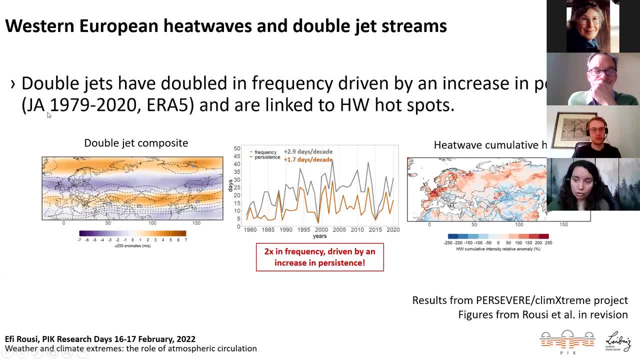 found to increase. we're talking about July and August, the summer months and the period of the reanalysis data data set era five, from 1979 to 2020.. And we see that those double jet days have increased both in frequency and persistence, And this increase is driven by the 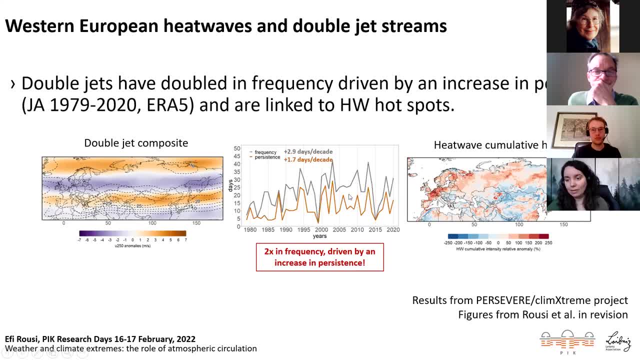 increase in persistence. So we have more consecutive days of double jet occurrence And if we look at the composite of the double jet days regarding the cumulative intensity of heat waves compared to climatology, we see hotspots in different regions of the Eurasian sector. 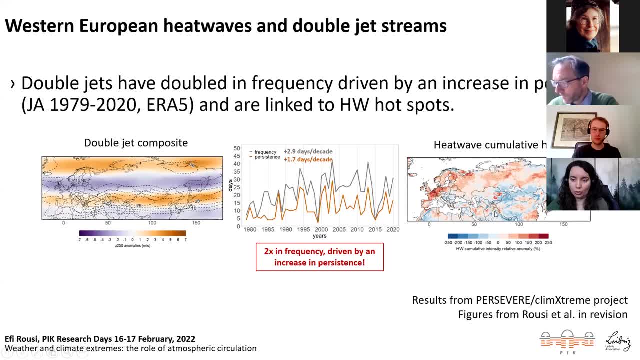 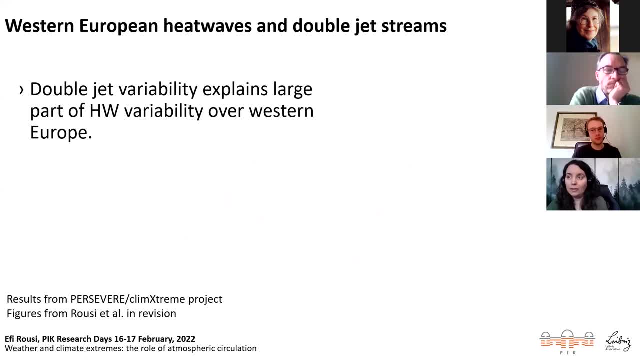 But most importantly here over Western Europe. So then we wanted to see whether this double jet variability can explain some part of the heat wave variability over Europe, And we applied the linear regression model And here we see the results. So here we see the explained heat wave variance by the double jet variability. 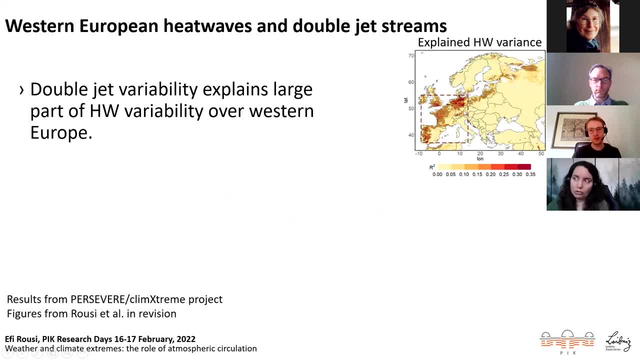 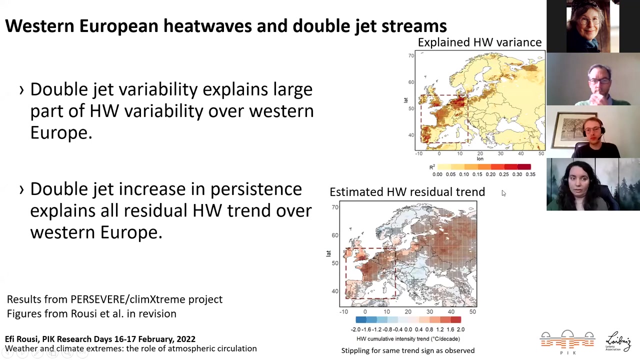 And we see that all the dots that we see in many grid points over Western Europe are statistically significant and the explained variance in Western Europe reaches up to 35%. Then we wanted to see whether the increase in the double jet persistence that we found can explain some of the heat wave trend in Europe. And here we saw the estimated heat wave trend. 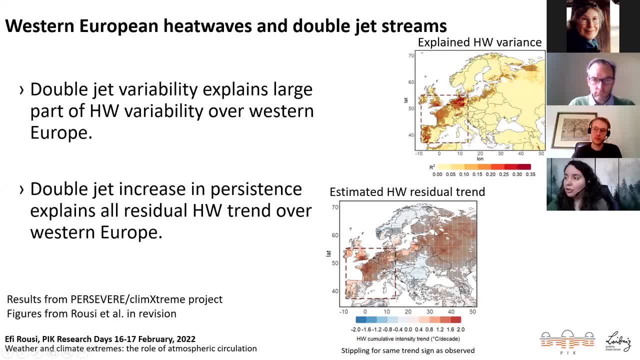 based only in this increase in persistence of double jets. So all the grid points that have dots now mean that they have the same sign of trend as they observed. So we see that this is the case for large regions of Europe, And if we aggregate over the whole European domain, then almost 30% of the trend can be explained by this increase in persistence of double jets. 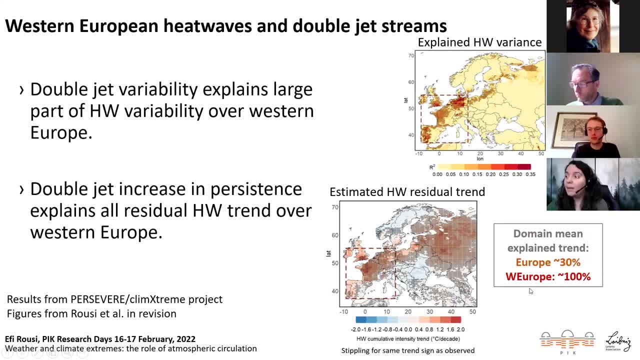 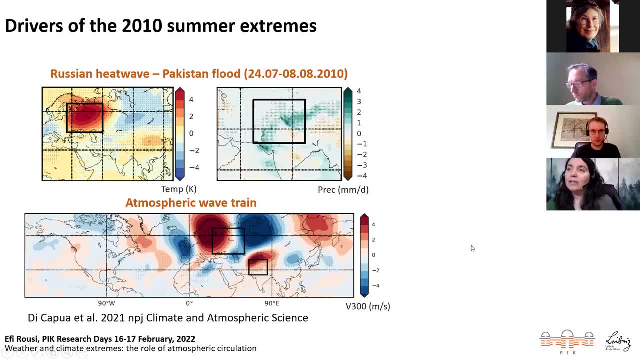 While if we focus only in this smaller part of Western Europe, this reaches up to 100%, which is a very important finding. And now we'll go a little bit further back and show you some results of our study led by Georgia DiCapua. 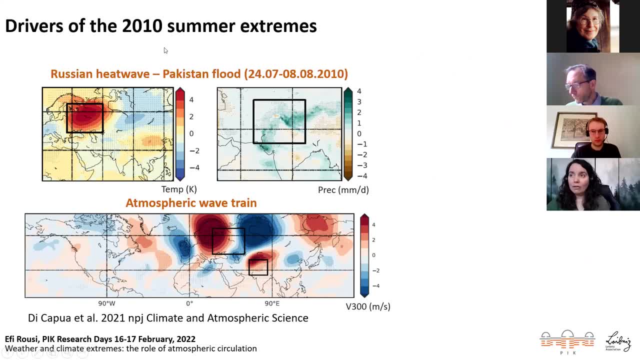 which was published late last year on the drivers of the 2010 summer extremes, And again, this summer was very characteristic because we had contemporaneous concurrent extremes- the Russian heat wave and the Pakistan flood- which were actually linked by an atmospheric 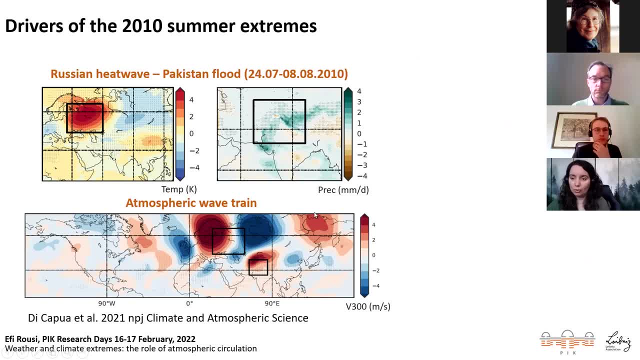 wave trend, So an atmospheric wave trend in the upper troposphere, a succession of highs and lows, practically but connected to the true extremes. In this study, we looked at the large ensemble of a modeling experiment for summer 2010, in order to try to calculate the contribution. 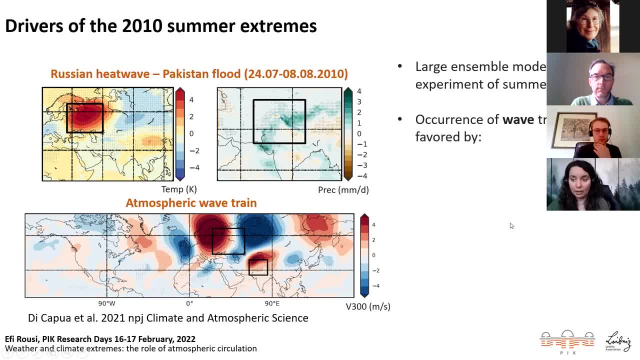 of different factors to the occurrence of this atmospheric wave trend, And three factors were important in favoring this wave trend. First, sea surface temperature anomalies over the globe. In particular, this year was characterized by a strong La Nina phase in the Pacific Also. 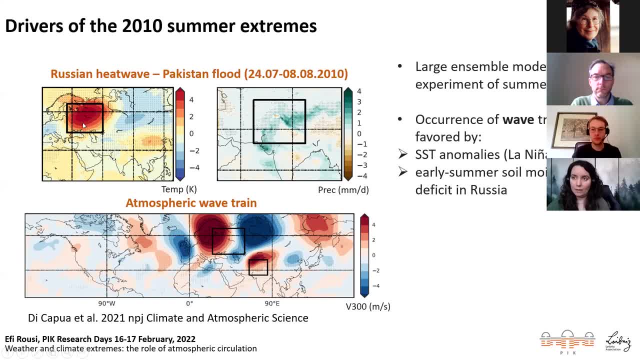 early summer soil moisture deficit in Russia, more or less in the same region of the heat wave, was important And, most importantly, high latitude land warming. So here when we talk about high latitude, we mean above 65 degrees north, And this is important specifically for our research. 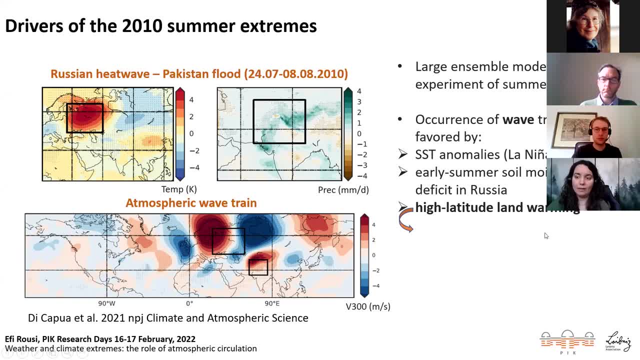 because this high latitude land warming, which is part also of the greater Arctic amplification that we know it has to do also with the weakening of it, results actually to a weakening of the jet stream and the storm tracks And also it seems to be favoring double jet states. 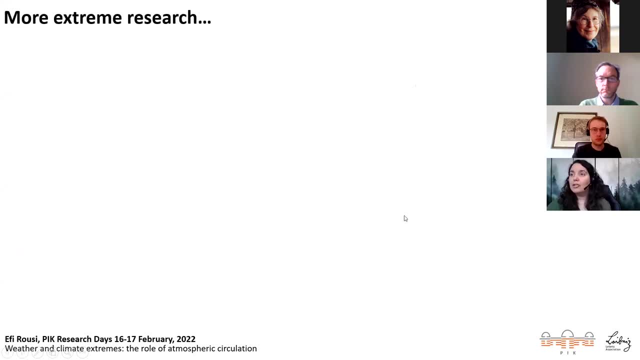 like the ones that I discussed before. So I have one last slide with some very- I will very briefly refer to other research that we are doing in the group. So we have been also looking at the AMOX slow down and the consequent North Atlantic cold. 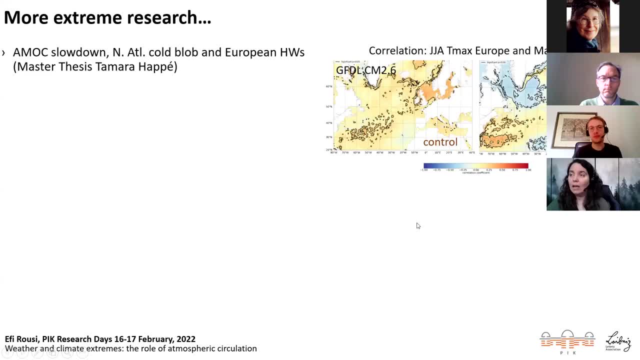 blob and their links to the European heat waves, Because we have seen in some observational studies recently that some important heat waves like 2015 and 2018 were preceded by particularly cold North Atlantic sea surface temperatures, And our student, Tamara, looked at this in a model. 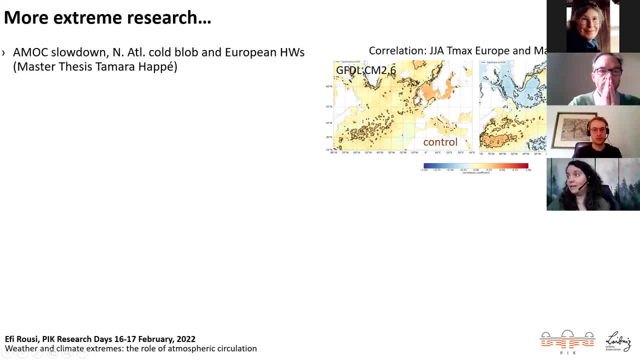 and found that, under a doubling experiment, indeed, summer temperatures over Europe are preceded by this cold May, since the warm temperatures are so high that for the cold summer we are seeing a much higher rate of snowfall than for the tropical winter in the South Atlantic. And the reason we look at that is because we have seen that, you know, the temperature has increased rapidly And the reason is that, if we look at, the heat waves had a great impact on the entire Arctic. there is a very important heat wave And so, regardless, we are also looking at the North Atlantic cold and the heat waves have a great impact on 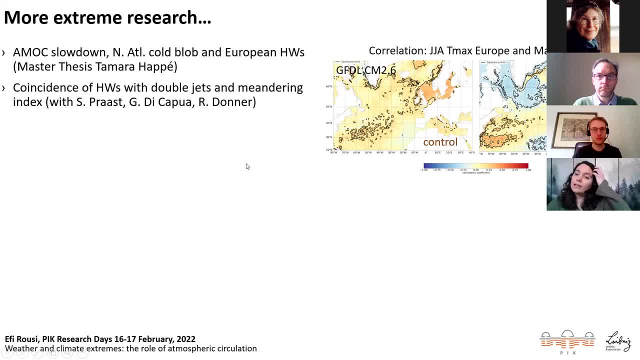 sea surface temperatures. Other topics we have been looking at are coincidence analysis of heat waves with double zeds and also the Mandarin index, which links to previous work by Georgia and together with Tim Kaumau, And we have been also working together with Johanna Beckman from the Ice Dynamics Group and have been 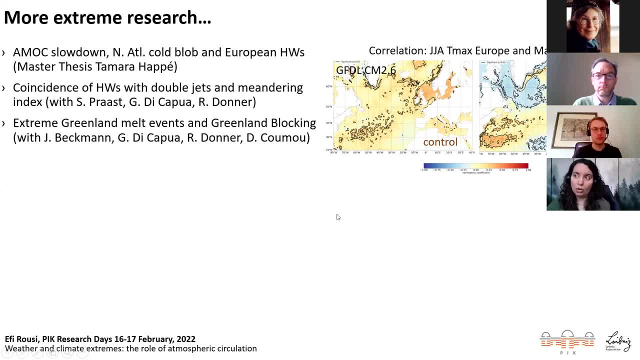 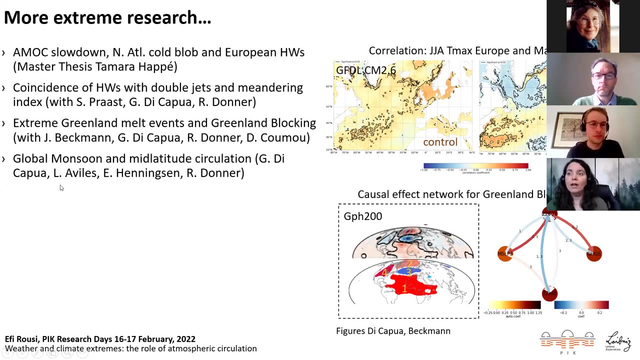 looking at the Greenland melt events and the links to Greenland blocking. I will not go into details but this is just an example of a causal effect network for Greenland blocking index. And last, Georgia Di Capo is also continuing her research on the interactions of the monsoon, both the Indian and the